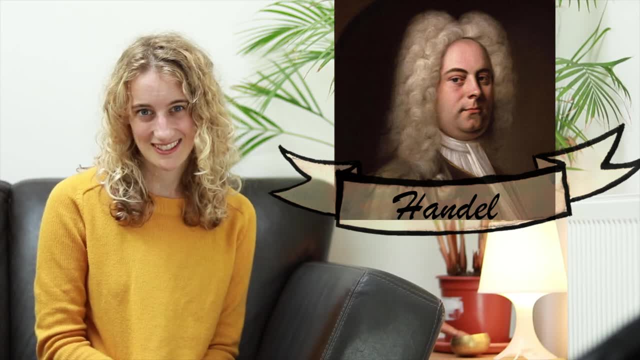 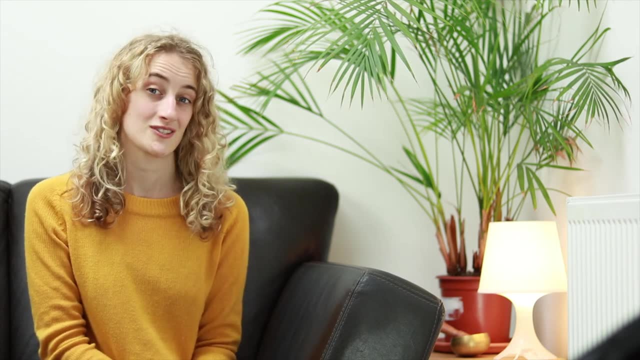 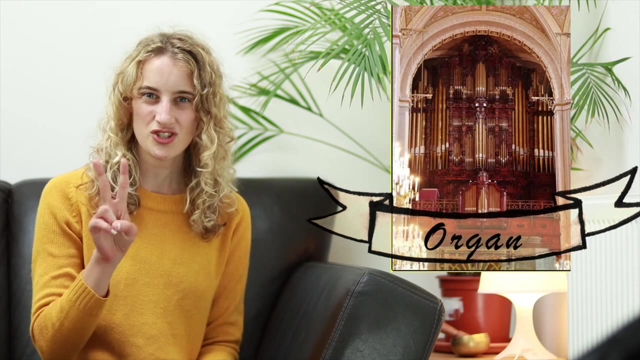 and Handel. In the Baroque era, instruments were different from today, which meant that they had very different timbres. Instead of the piano, harpsichords were commonly used, as well as other music organs which had two different sounds. Even stringed instruments were different. They 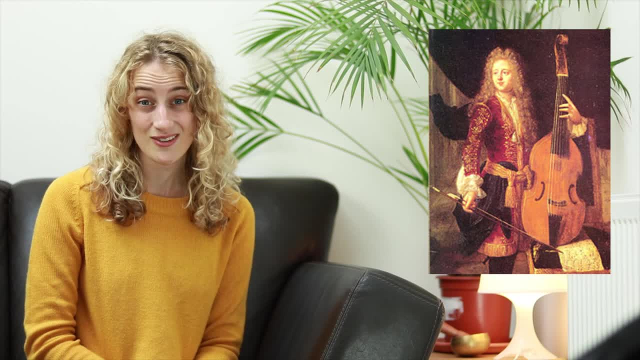 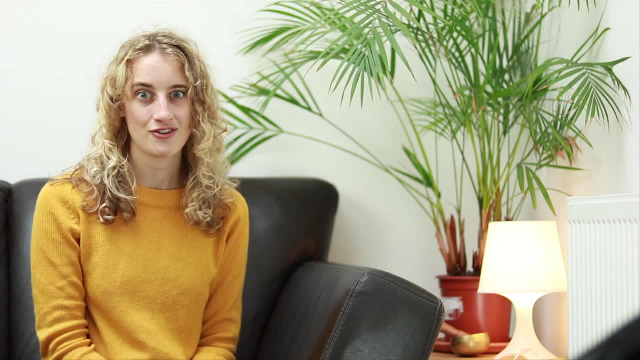 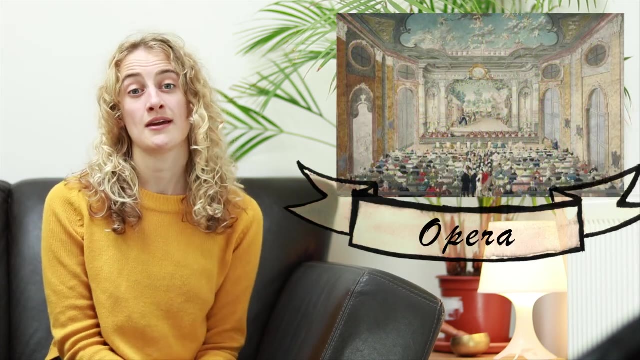 were made with gut strings rather than steel strings, which gave them a very different sound. Now, lots of new types of music were being created In the Baroque era. opera became popular Before the Baroque period. in the Renaissance era composers often wrote polyphonic. 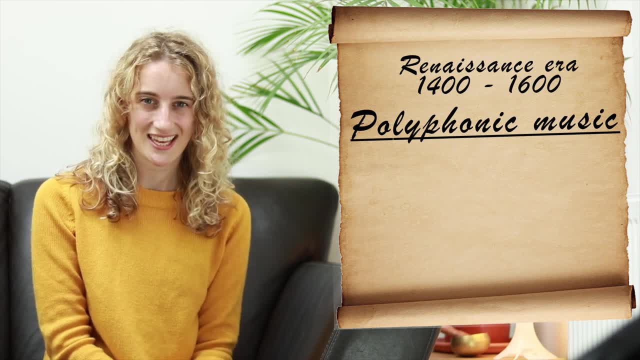 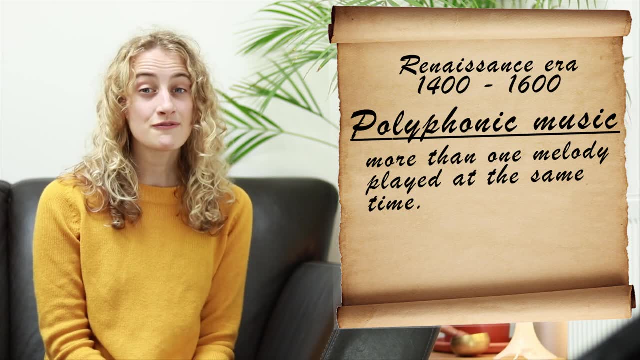 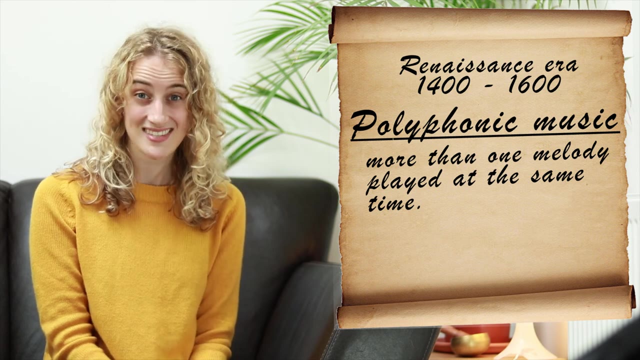 music. Now, polyphonic music is when more than one melody is playing at the same time. In fact, it was very popular in the Renaissance era for lots of different vocal lines to be happening at the same time, with different rhythms and sounds. 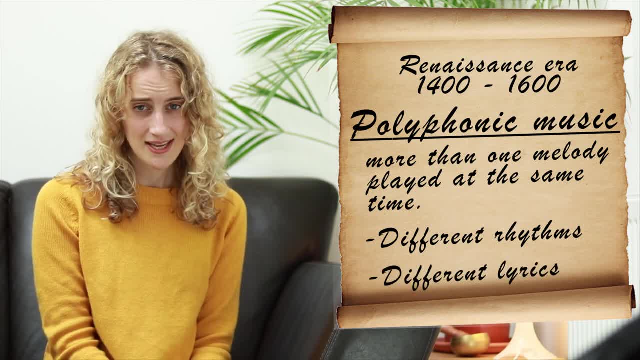 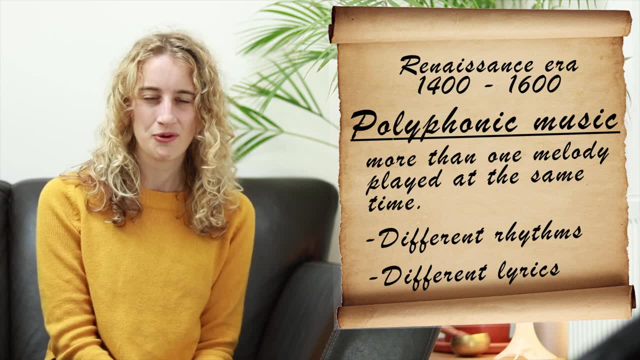 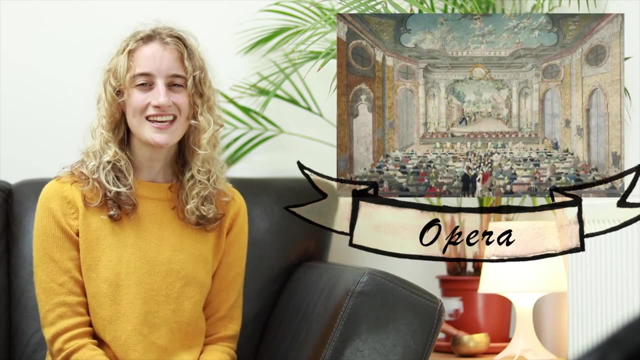 So it was very popular. So it was very popular. There were sometimes even different lyrics. You can hear a lot of this in Renaissance church music. It wasn't so important for the audience to be able to hear what was being sung about. However, in opera, the audience need to know what the singer is singing about. 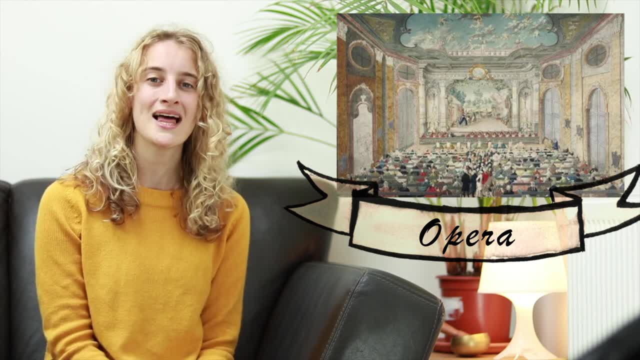 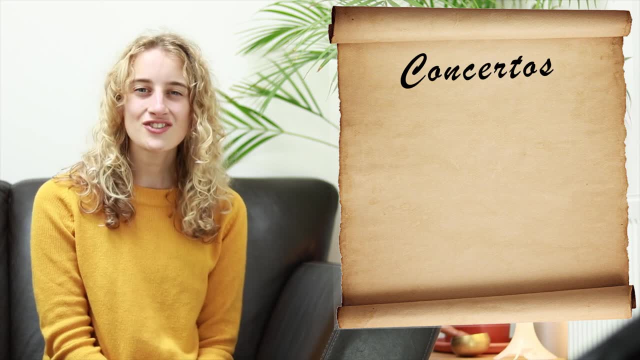 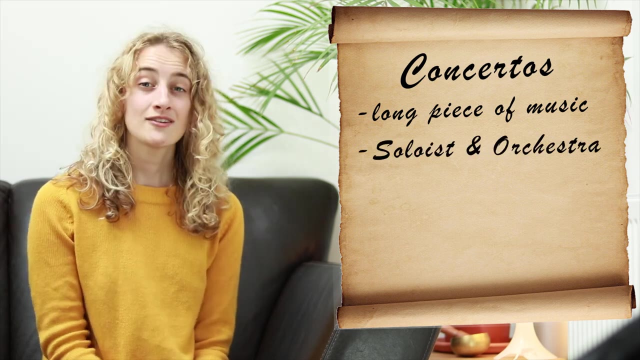 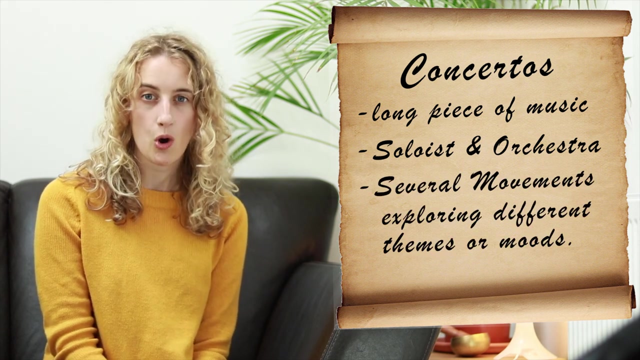 And so composers began to use melody and accompaniment. Now composers also began to write concertos. A concerto is a long piece of music written for a soloist and an orchestra. Now concertos are made up of lots of movements, and each movement explores a different theme or mood. 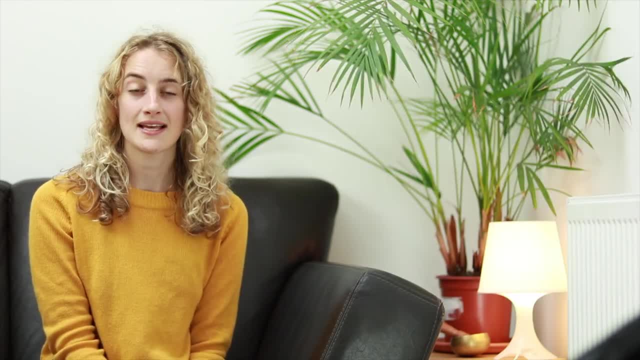 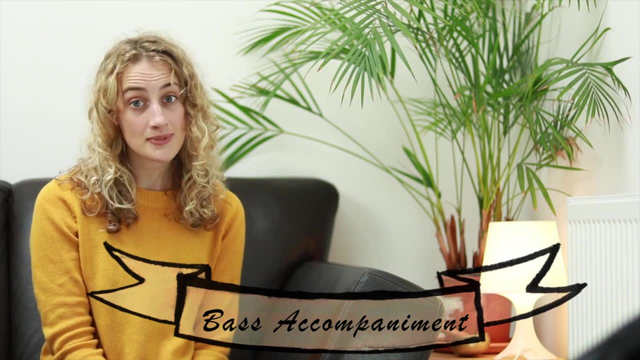 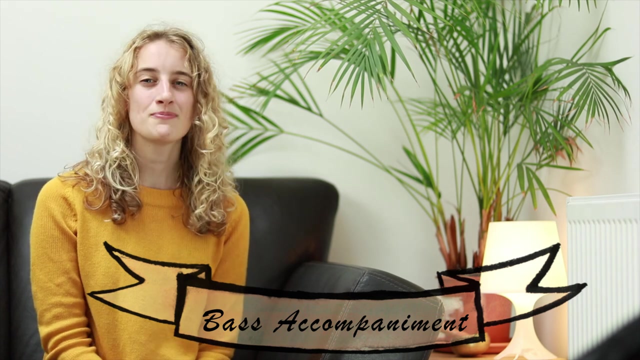 Music written in the Baroque era often has a melody and a bass accompaniment on an instrument such as the cello or the harpsichord Now, often Baroque composers would write a melody in the bass line in full, which meant that the bass musician would improvise the chords. 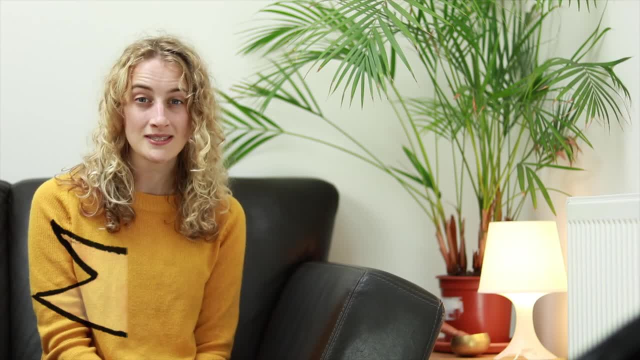 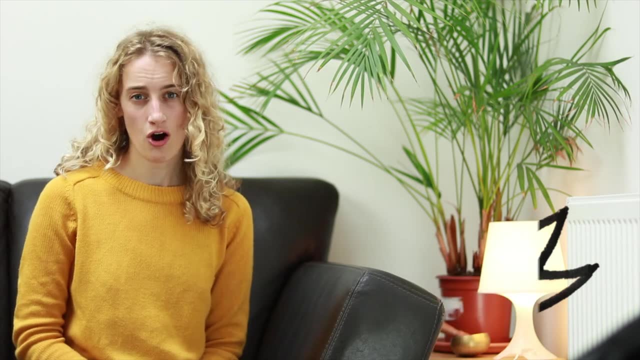 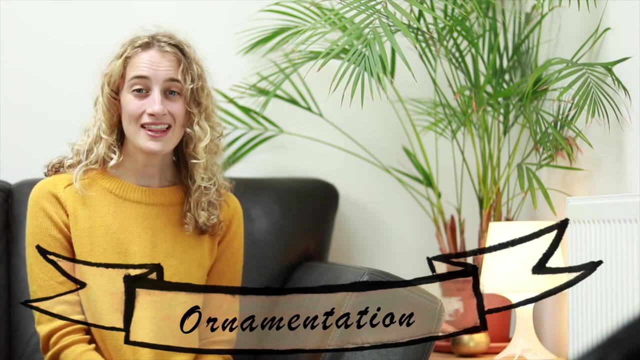 and the melodies that they played, And this is called basso continuo or continuous bass. Now, the melody in Baroque music often uses ornamentation. Now, this is when the composer writes the melody and the musician is free to improvise around the notes and the melody. 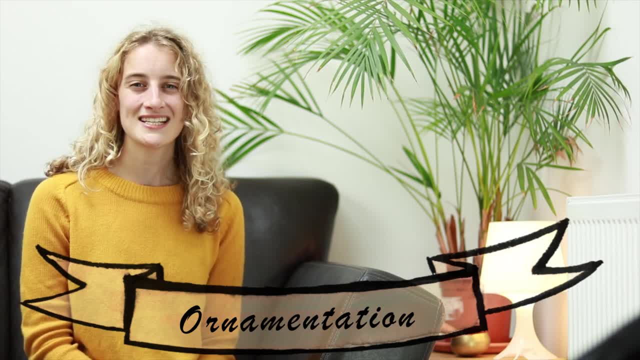 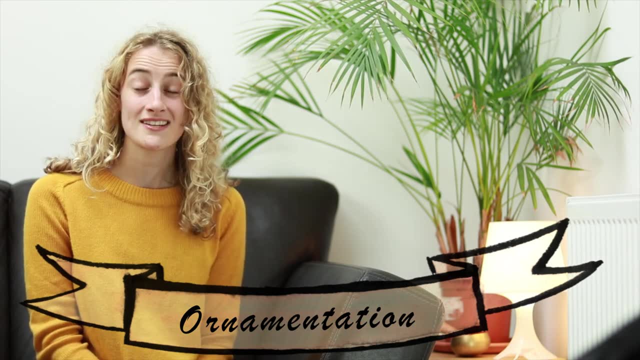 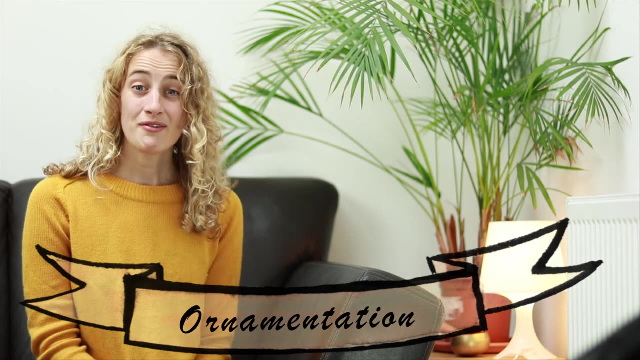 While making sure that the melody stays in time with the rest of the music. Nowadays, ornamentation tends to be written into the music, but in the Baroque era it wasn't always written by the composer. There are lots of different types of ornamentation. 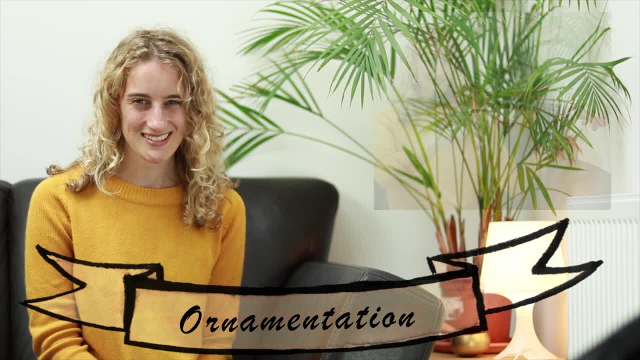 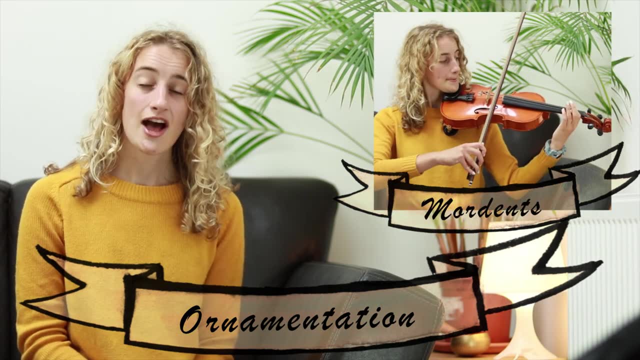 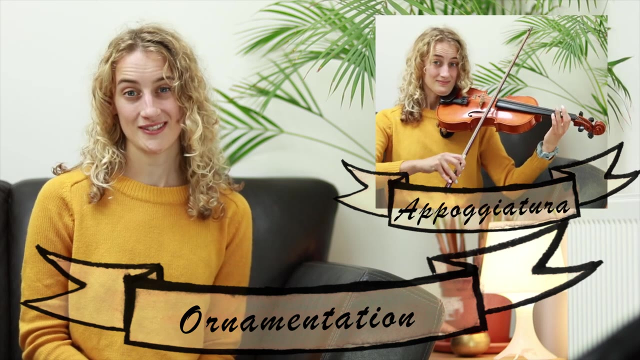 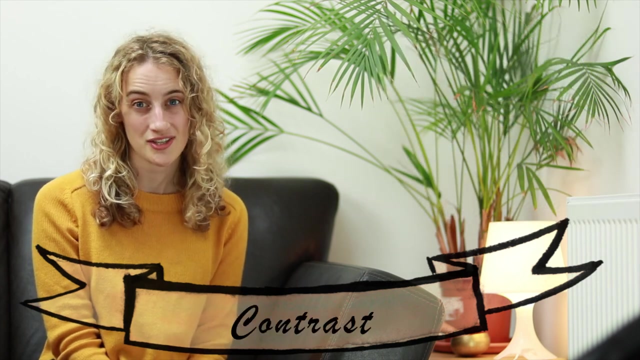 One of the most popular kinds is called a trill and it sounds like this. You can also have mordants, terns and grace notes, appoggiaturas and acciaccaturas. Another feature of Baroque music is contrast. Composers often contrast, whether it's dynamics. 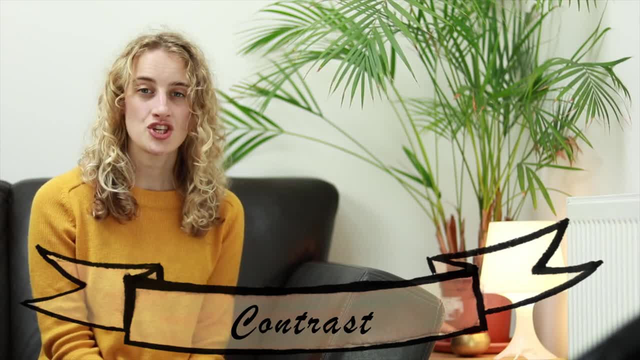 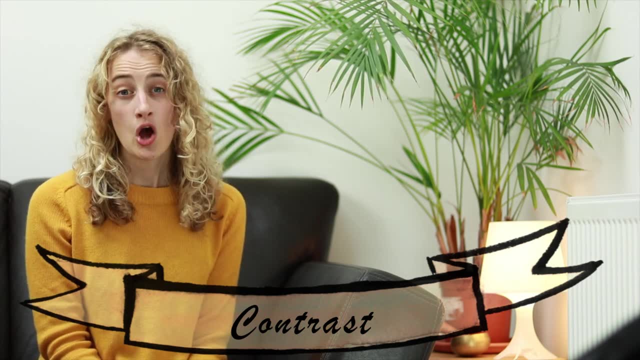 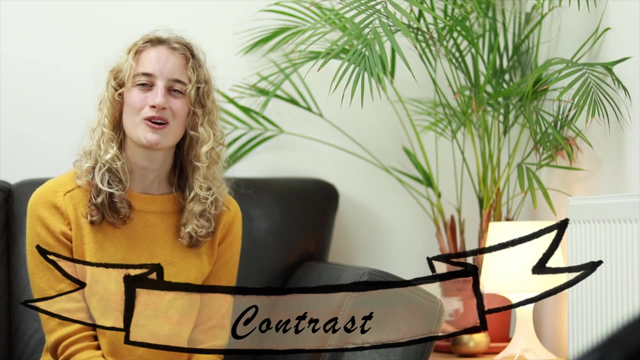 loud and quiet timbre by changing between instruments or going from a soloist to a duo or aero or an ensemble, or going from one instrument to multiple instruments. Now let's listen to a piece of Baroque music now, and I want you to listen for all of those. 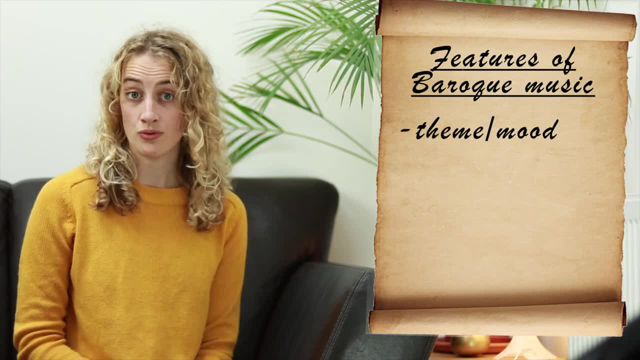 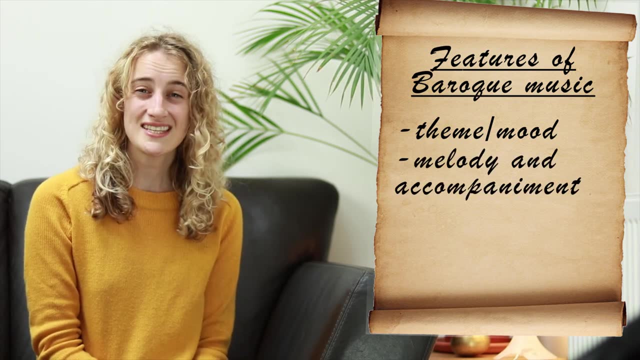 different features that we've talked about: The mood: what do you think the mood of this piece of music is? Listen out for a melody and accompaniment. See if you can hear the basso continuo, continuous bass line. See if you can hear some ornamentation that is slightly off key and sounds like this: